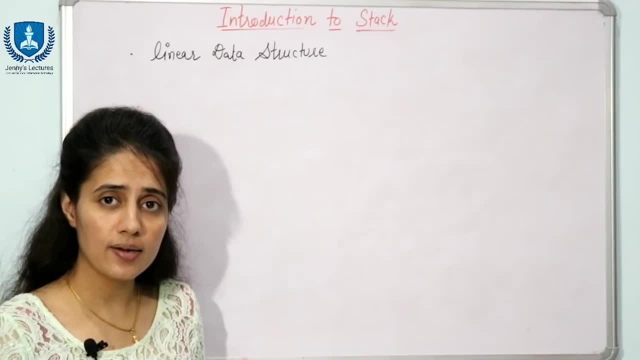 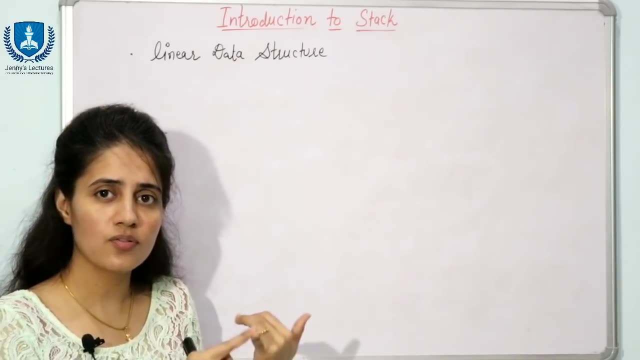 Data right. We have discussed few data structures like array and linked list: How data is stored in array. What are the different operations on array. What is linked list? What are the different operations on linked list, How data is stored in linked list. right, And now we will see what is. 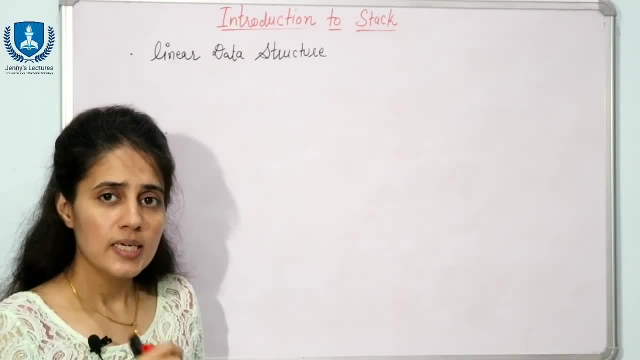 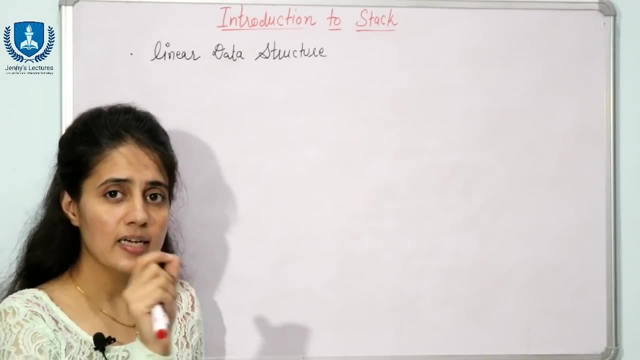 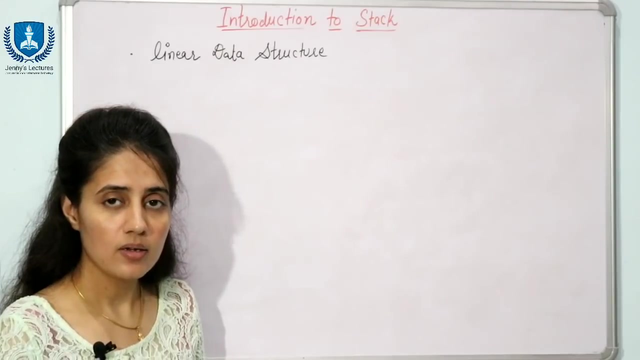 stack data structure. So you can see it is a linear data structure, fine. And see in array what is there? Random access is possible. You can directly access any data in a constant time In linked list. what? Only sequential access is possible, right. What about stack? In stack only. 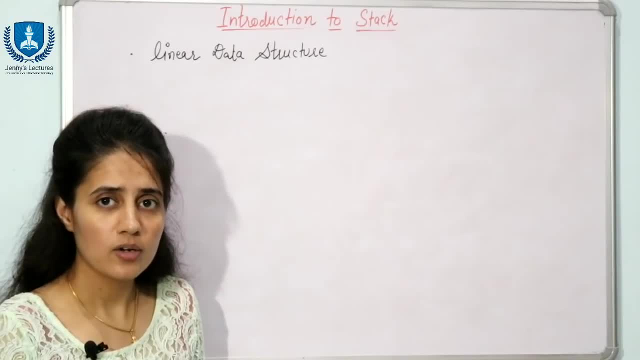 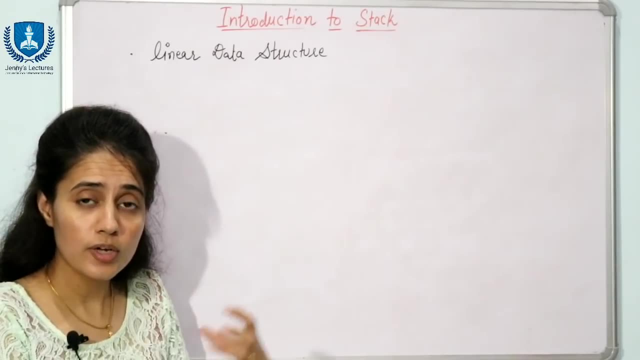 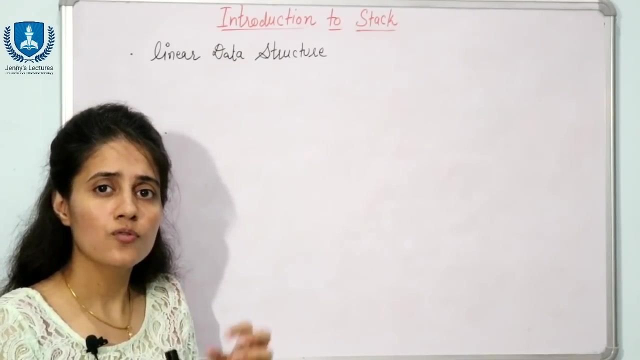 you can say limited access is possible, right? Or you can say it is a ordered list. What is stack? It is an ordered list. or you can say it is a collection. or you can say it is a container which is going to follow a rule for insertion and deletion of the data, right. 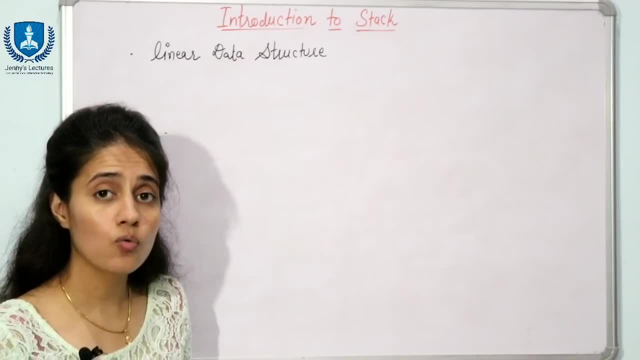 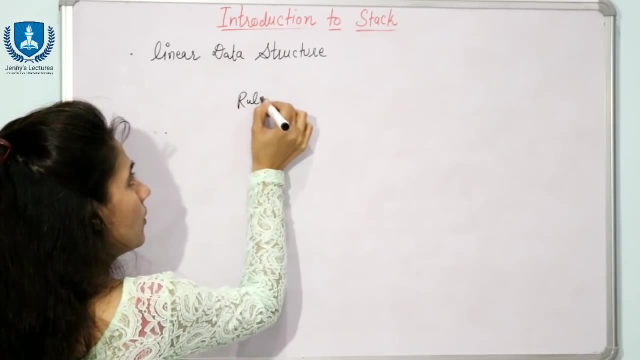 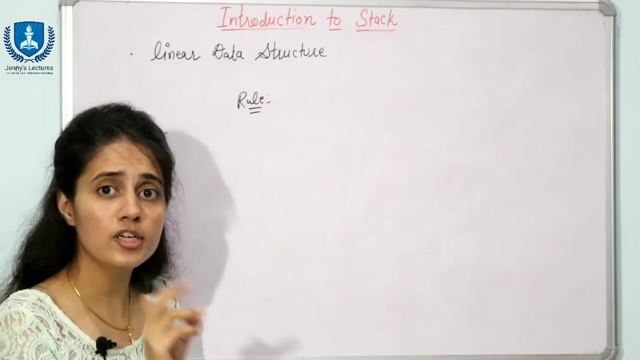 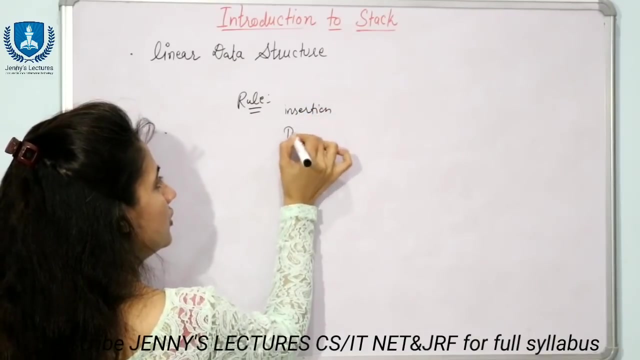 Right, and what is that rule or what is that restriction you can say, or what is that principle right, which that stack data structure follow? so that rule is: insertion and deletion is possible only from one end, right? this is applied on both insertion and deletion: insertion and 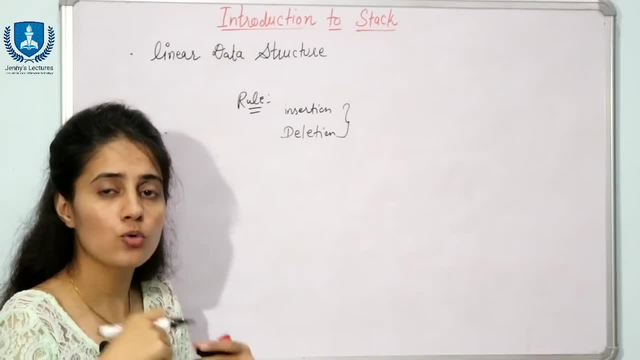 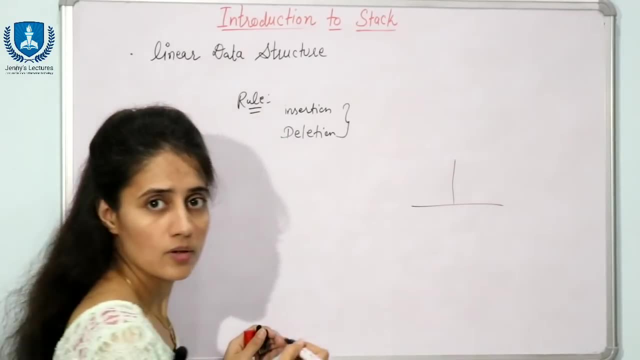 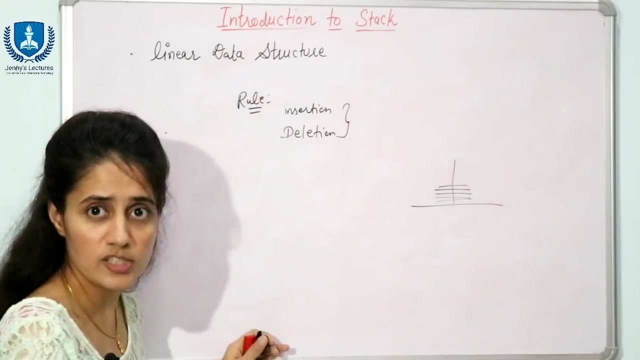 deletion is possible from only one end, like you can take a real life example: suppose you have a cd stand right like this: you are going to put cds here, first cd, then second, third, fourth, fifth, obviously. like this you are going to put: suppose you want to insert another cd. in that case you 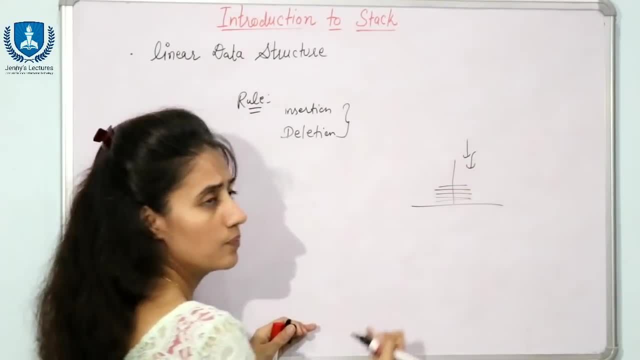 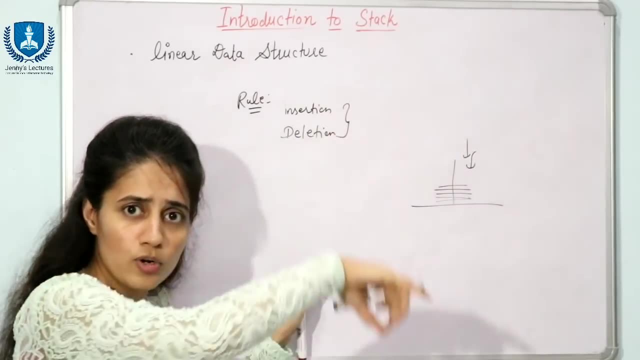 have only one way to insert cd: from the top only. you cannot insert cd here from the bottom. you can insert cd from the bottom. you can insert cd from the bottom. you can insert cd from the bottom. you cannot insert from the left or right. the only way is from the top only you can insert that cd. 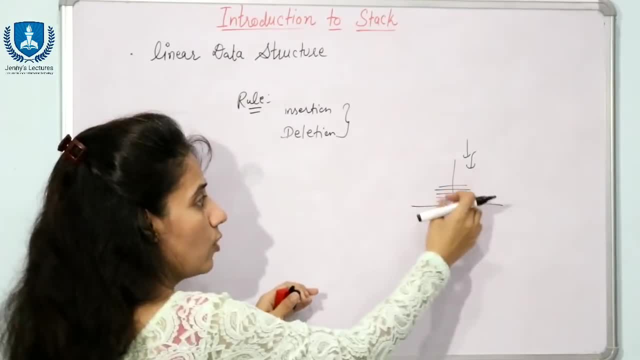 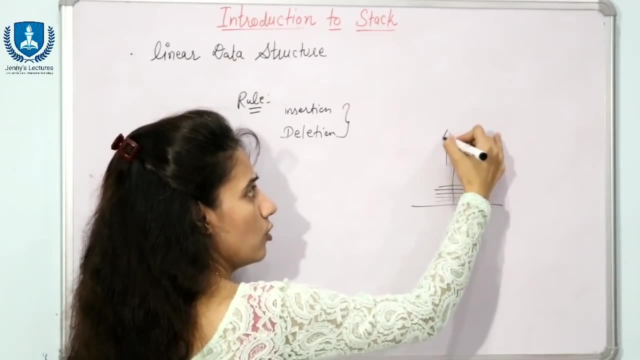 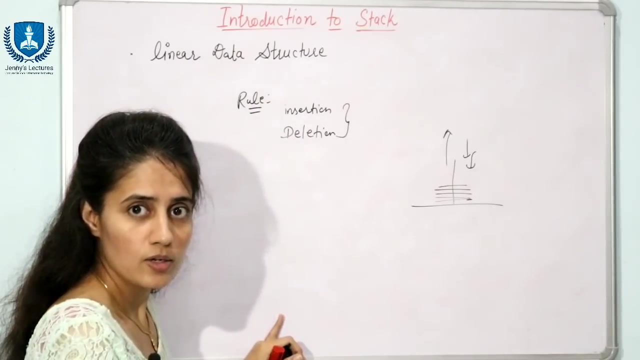 right. second case says: if you want to take out a cd from this cd stand, then what you will do, only one option you can take out from the top right. suppose you want to take out this cd, the first cd, right? so you don't have any option. the only option is: first of all you will have to take 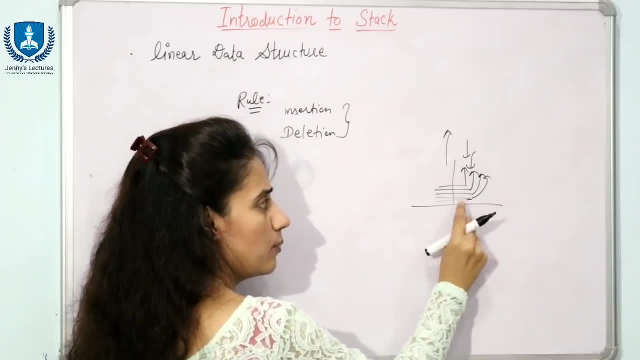 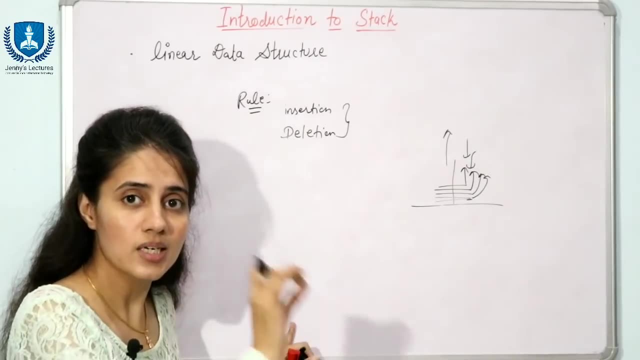 out. all the cds with the cd stand right, so you can insert cd from the top. only you can insert which are placed above this cd. after that, only you can take out this cd, right. that is the restrictions on insertion and deletion in stack. fine, so in this video we will see how logically 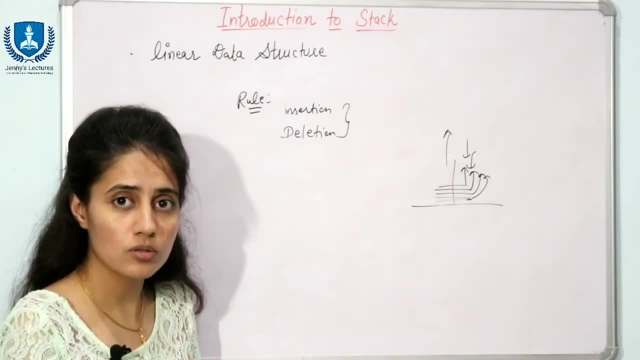 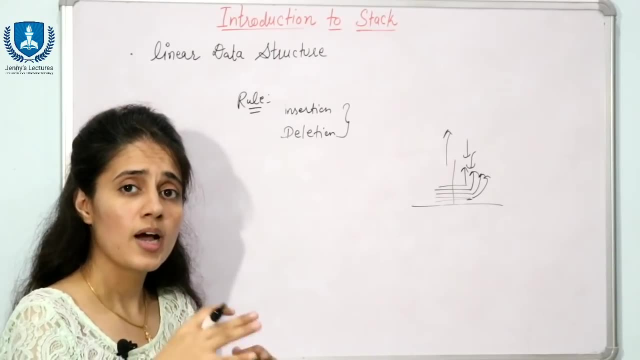 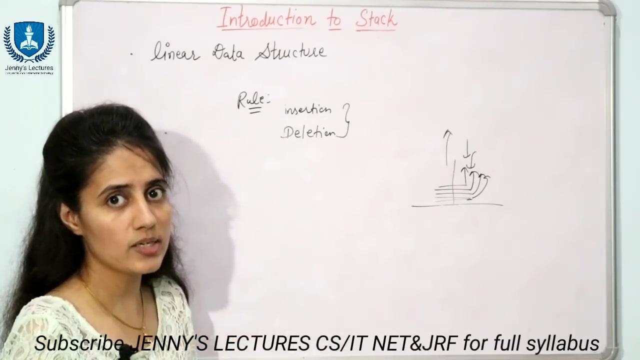 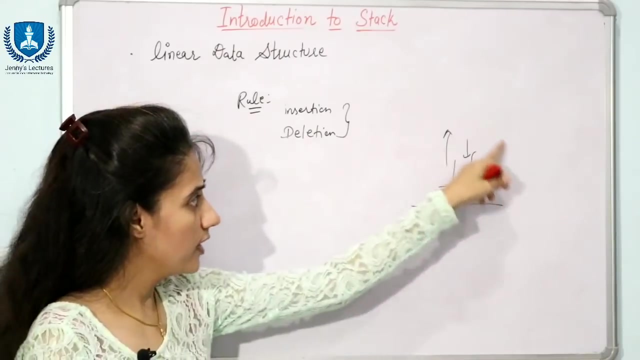 you are going to represent a stack. what are the introduction, introductory part of stack, some basic operations on stack. what, what are the meaning of those operations, as well as some applications of stack. in next video, we will see how to implement a stack right using arrays as well as using linked list. so now like this: if you map this real life stack. 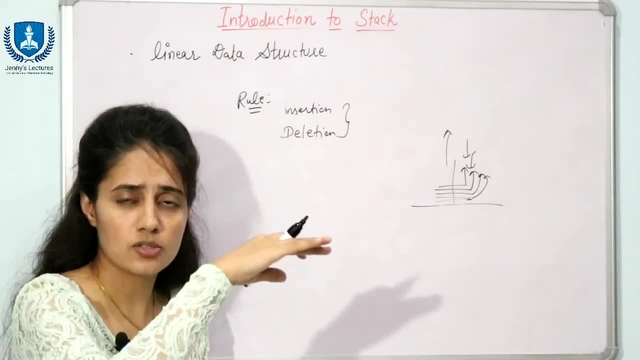 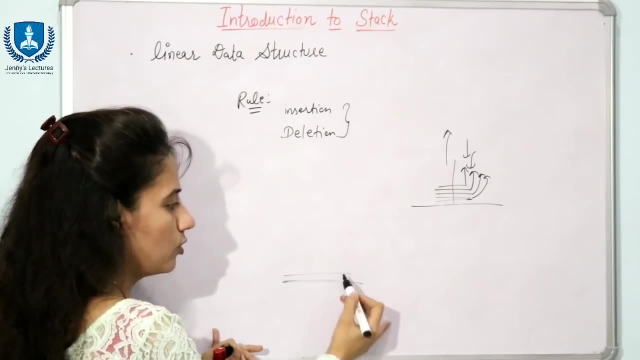 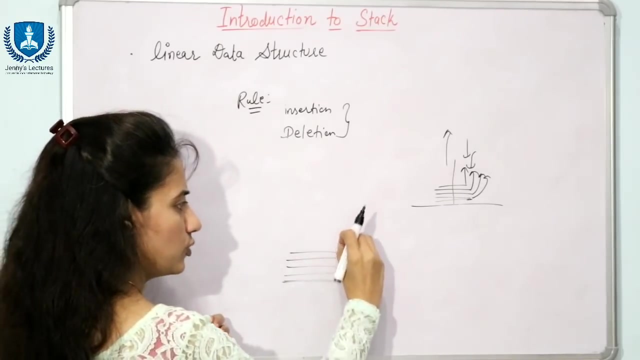 obviously this is what- a stack only, or you can say a stack of plates- right, one plate is. you have put one plate here. if you want to place another plate, then you will put on this plate, then third, then fourth, then fifth, like this you are going to place. if you want to remove a plate, then first. 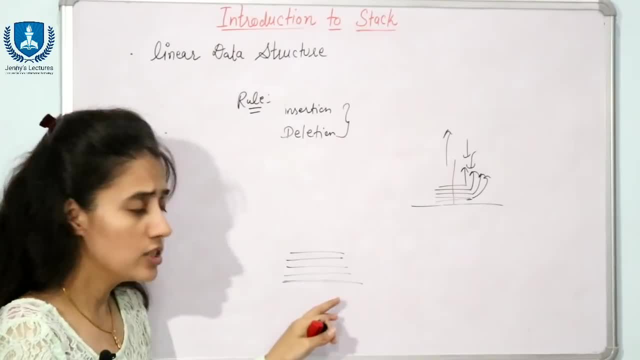 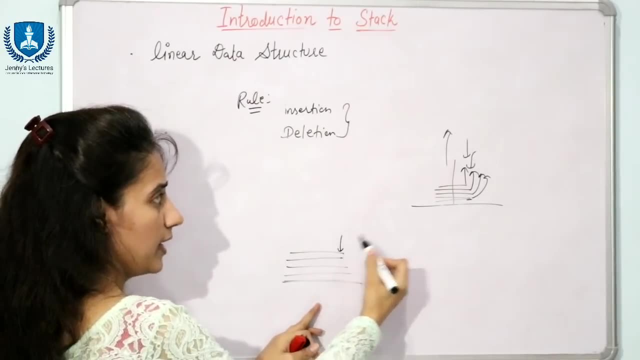 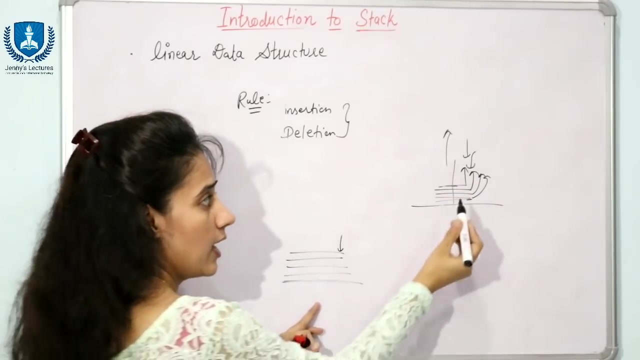 plate you will take out first, right. so the principle is, what last in, first out. you can say, right, this is the last plate. or you can say this is the last cd you have put in this cd stand, and the last cd would be the first one that you 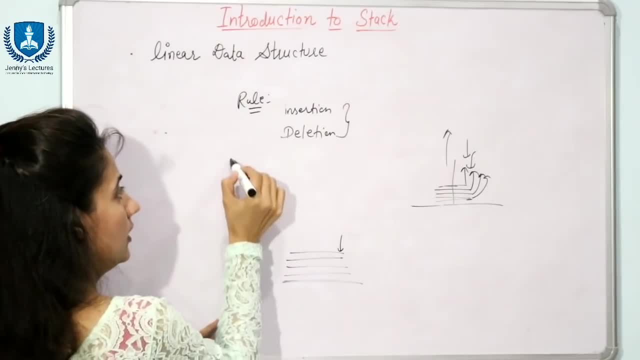 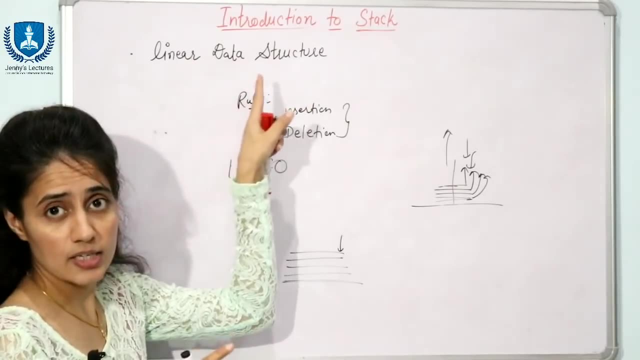 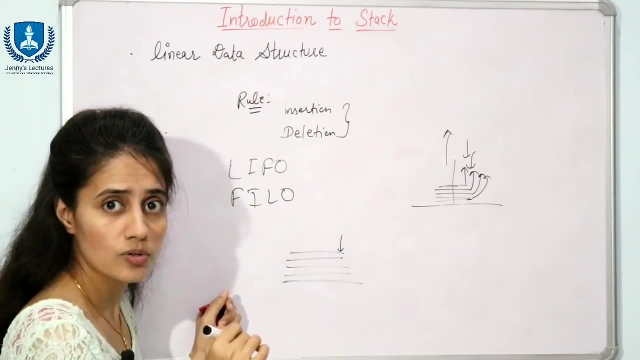 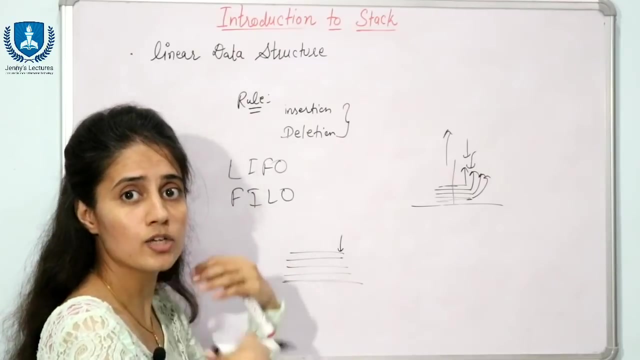 can take out. so last in, first out leaf over. so the rule on which this stack data structure works leaf over: last in, first out. or you can say first in, last out. this cd was first in, but if you want to take out this cd, then this would be the last one you can take out. because for for taking out this, 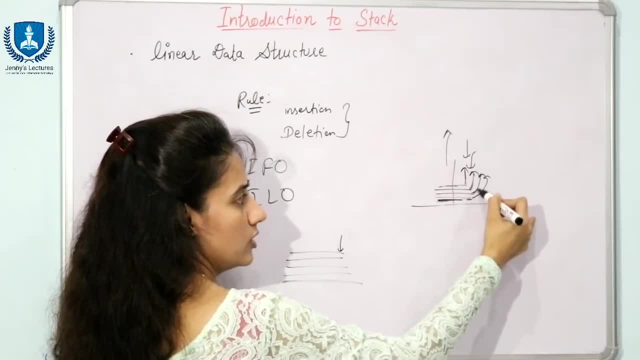 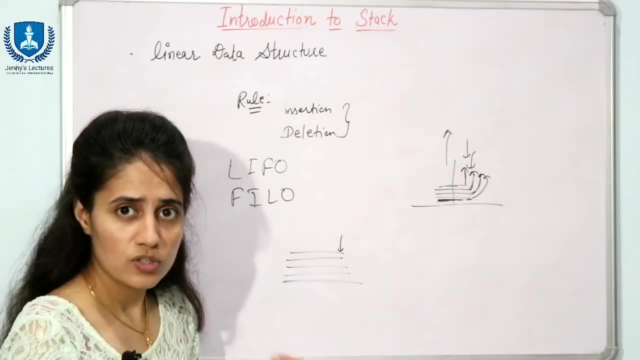 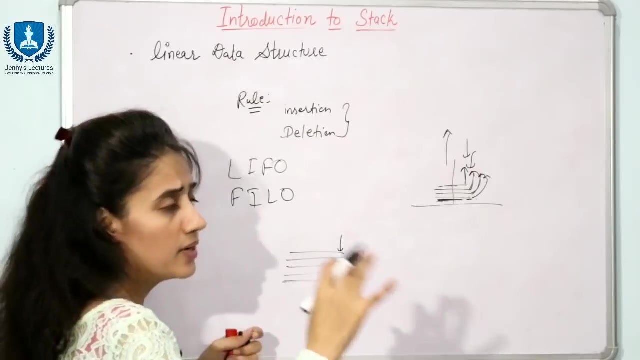 cd outside of the cd stand you have to take out all the above cds first of all. right, so first in, last out. and if you will map this real life example of stack in this with this stack, then you can say the logical represent representation of the stack is what we represent stack, something like this: 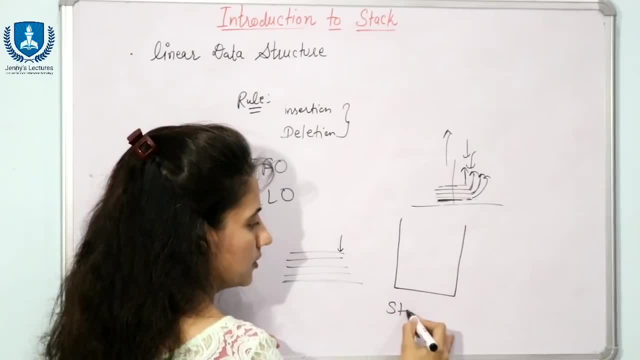 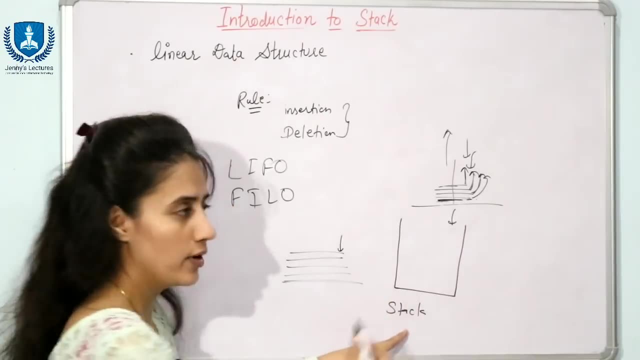 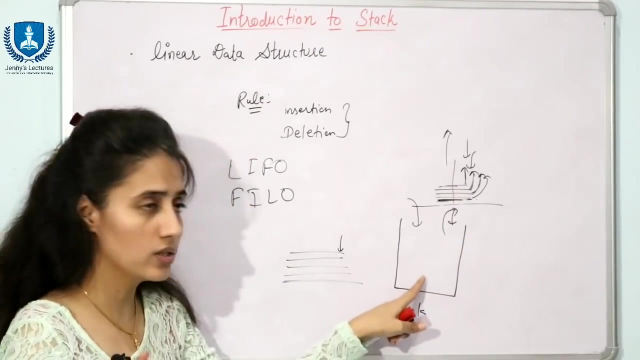 like this: this is what a stack you will represent this. it is a container which has only one open end. you can insert data from here. you can delete data from here, right. there is no other way. this is what a stack logical representation of stuff. this is not actual representation of stack, right that we? 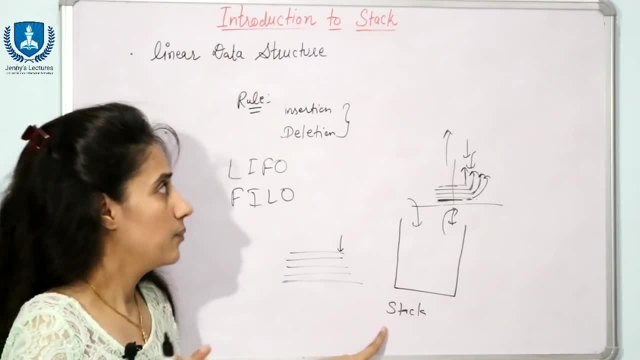 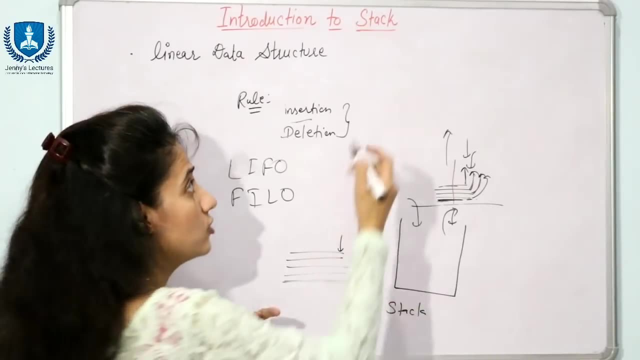 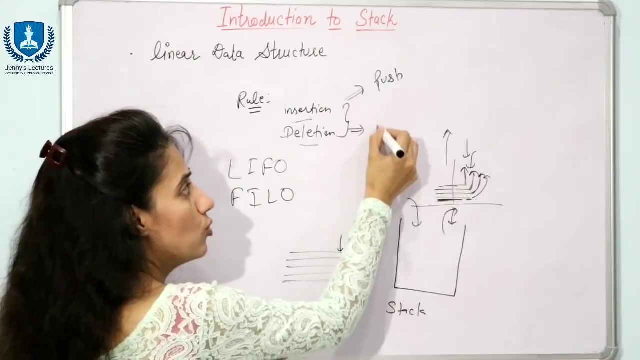 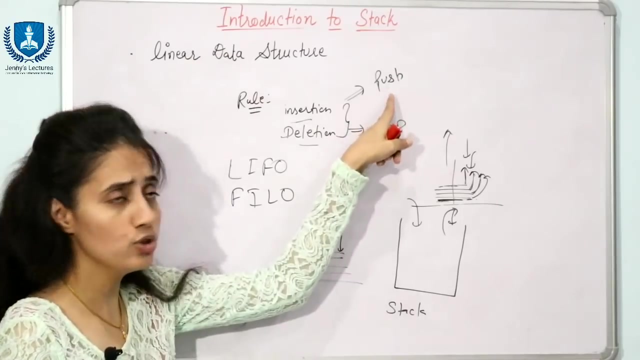 will discuss in later on videos right and in stack insertion operation, when you will insert some data in the stack. that operation is known as push right and deletion operation is known as pop. so two fundamental operations are there on the stack. one is push, one is pop. push means inserting or putting a data into. 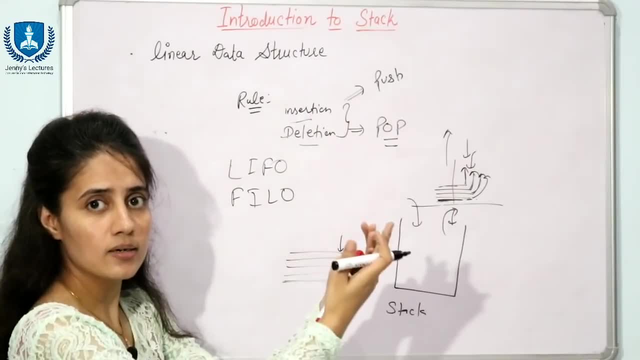 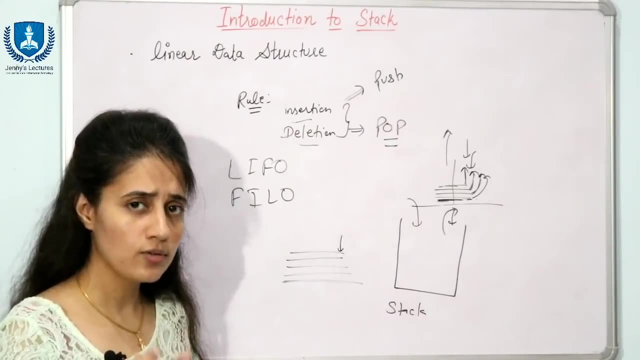 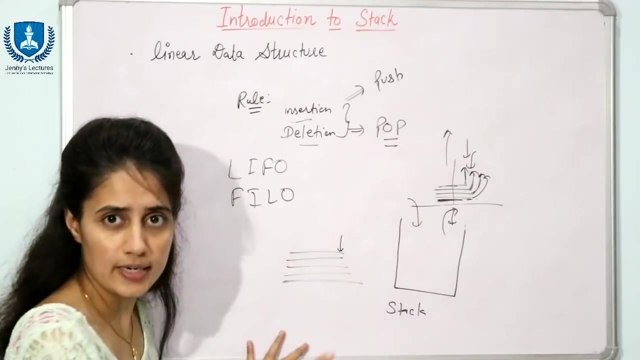 the stack. pop means push right, taking out or deleting the top most data from the stack right, two fundamentals operations. many more operations are also there that we are we will also discuss now. see, this is the only end from where you are going to push and pop the data right, so this is known as top top of the stack. 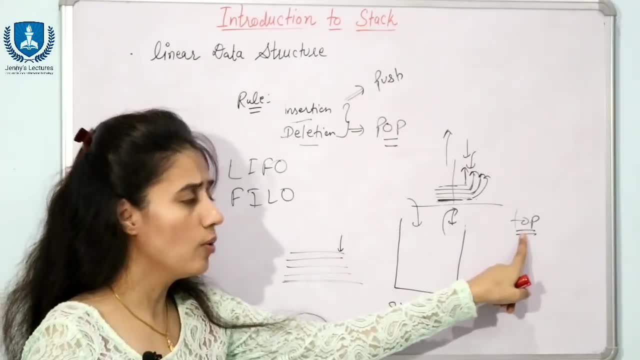 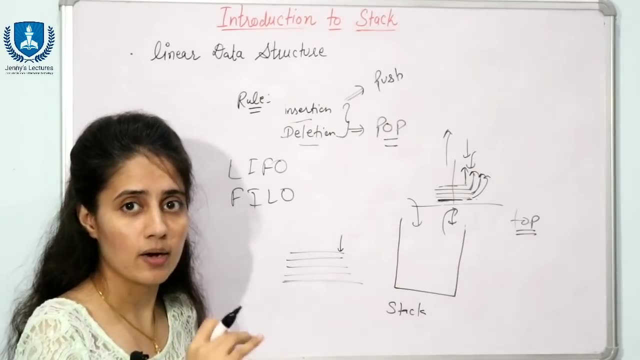 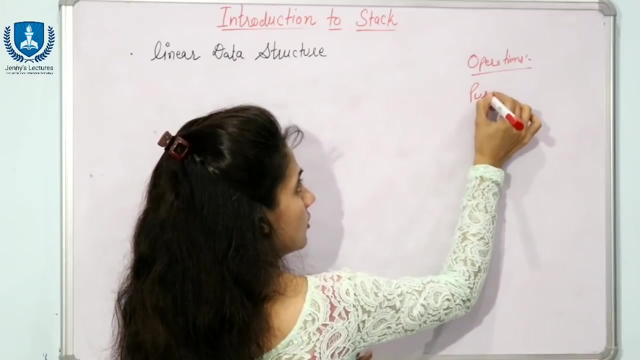 right. you can insert a data and you can delete data from top of the stack. that end is known as top, from where you can insert, you can push and pop data right. so now we will see some operations that are performed on stack data structure. see: first is push and in bracket you will write down. 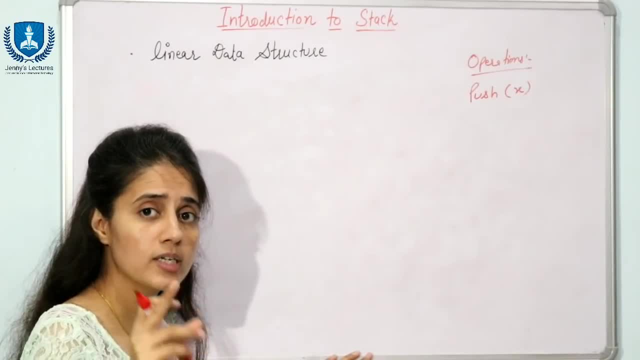 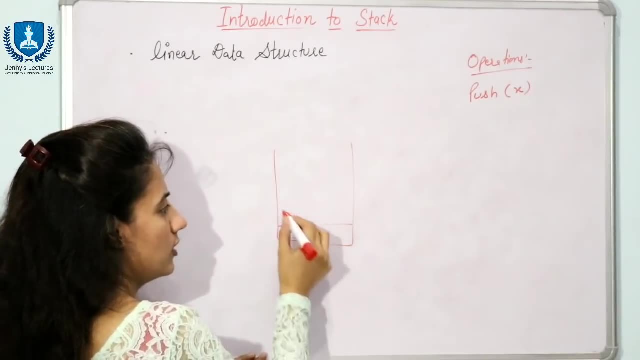 that data you want to insert into stack. see, stack is what it is: a collection of similar data type. only it's not like that. this is stack. and here the first data is suppose integer, and after that i'm inserting a character, after that, again, i'm inserting two. no, you can only insert the data of. 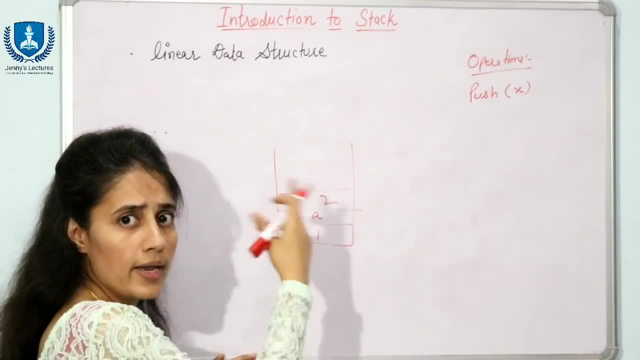 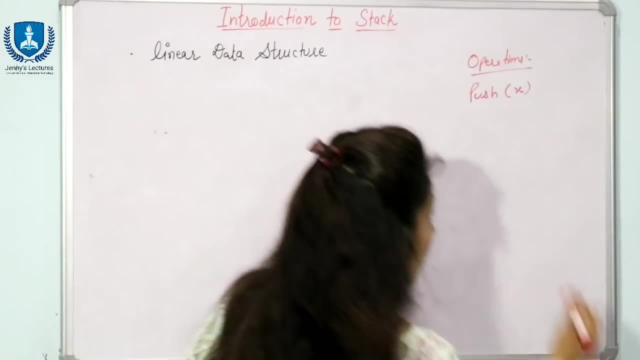 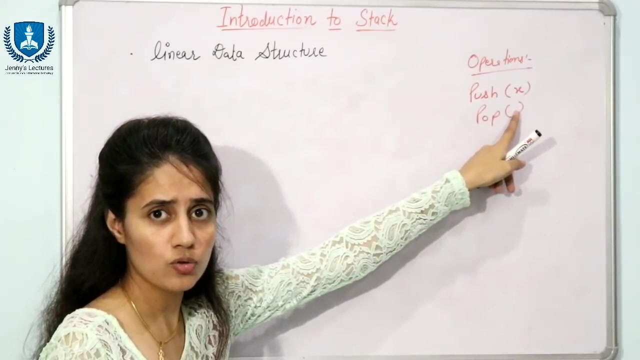 similar data type, either integer- all the data should be integer- or character or float, something like this: right see push. second operation is pop operation. right here. we don't pass any argument here. why so? because pop means always the topmost element would be popped out from the stack. 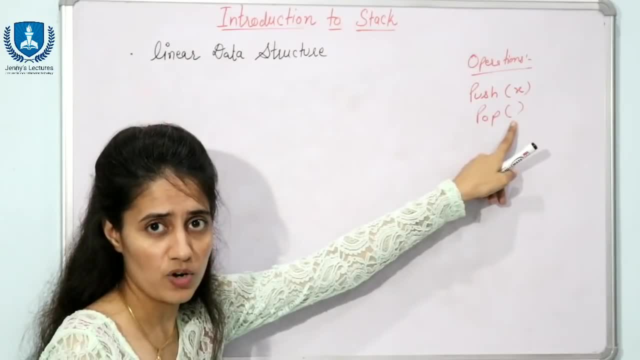 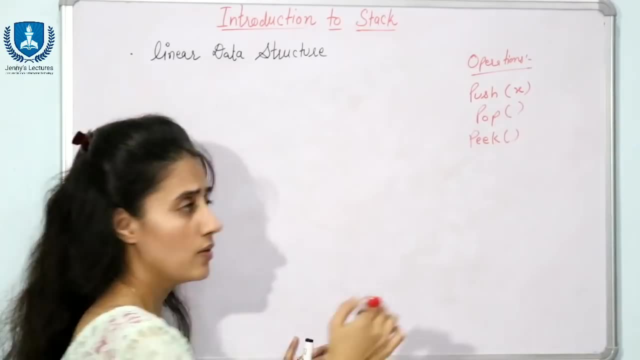 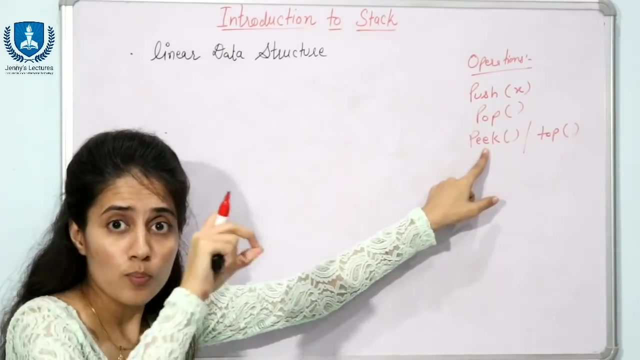 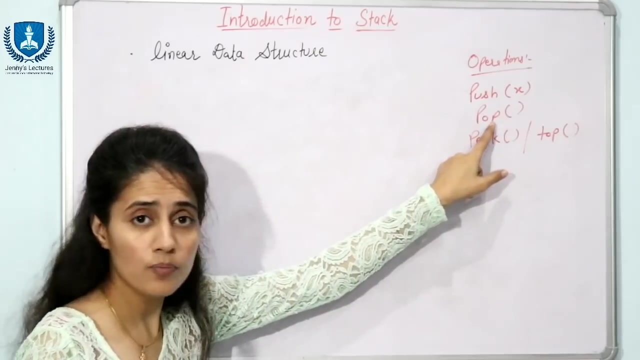 right, so no need to pass anything in this function. these are two fundamental operation. third operation may be peak operation or somewhere it is also known as top operation. it means what it is going to return, the topmost element of the stack, without removing that element from the stack. see pop will return. 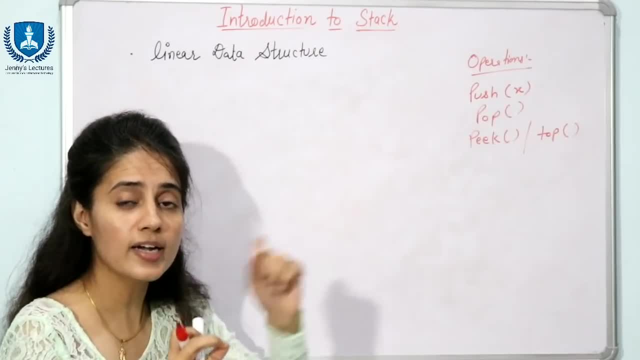 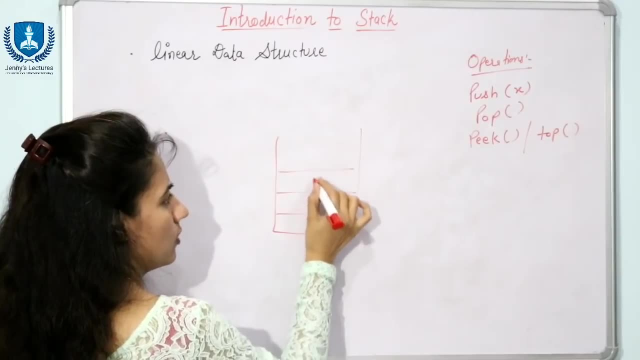 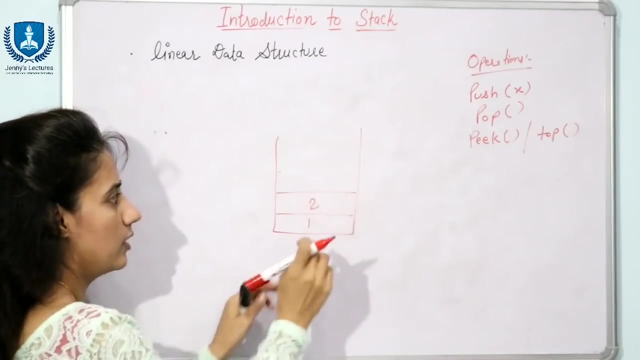 the topmost element from the stack as well, as it will remove that element from the stack. see, suppose this is what it is. i have stack and in this i have data type one. i have data one, two and three. if you write down pop, it means it will remove three from the stack. now, this is the stack, right and if and on this stack. 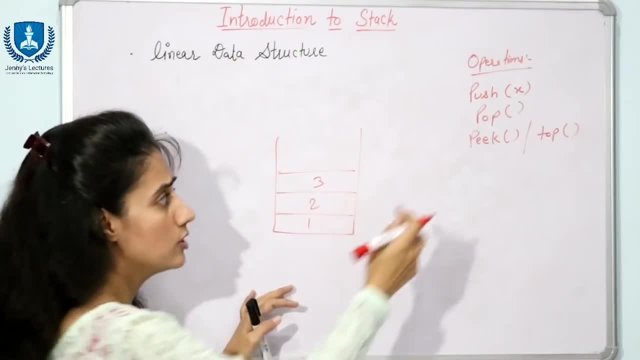 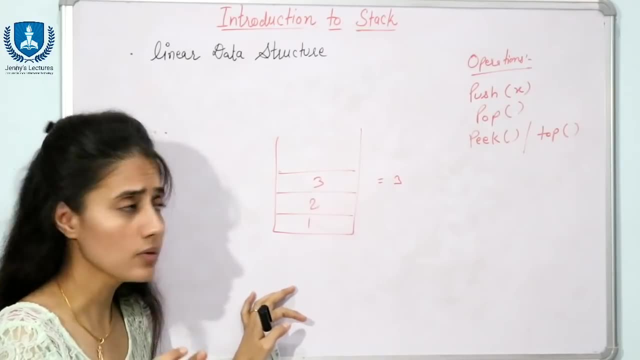 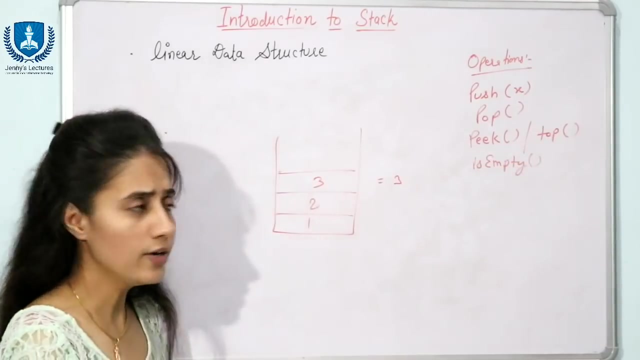 you will perform peak operation or top operation. it means it will return three, but it will not remove this from the stack. this is the difference. right? fourth operation may be is empty means it will true. if this stack is empty. there is no data in the list it has in the stack. 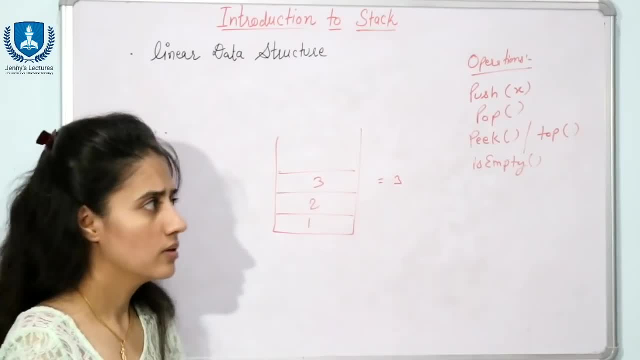 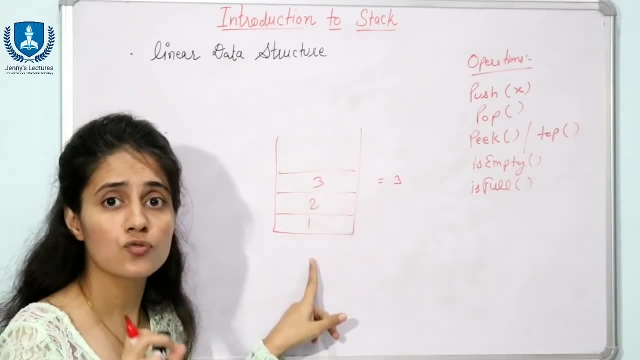 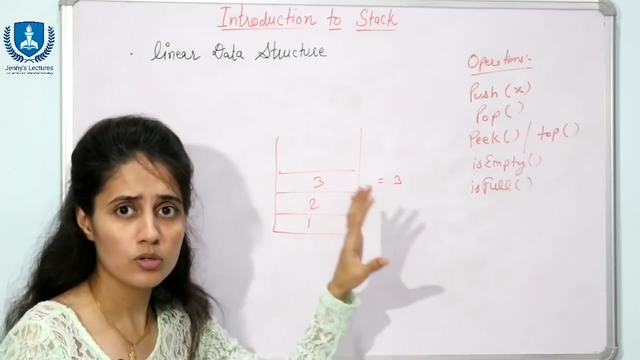 right, otherwise it will return false. another may be is full, so this function will return true if this stack is full. otherwise it will return false. see, these are not the only operation you can perform. there are many more operation you can perform on stack, like having array allows to perform important. 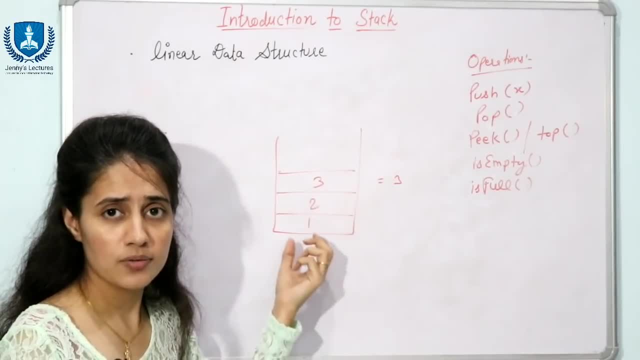 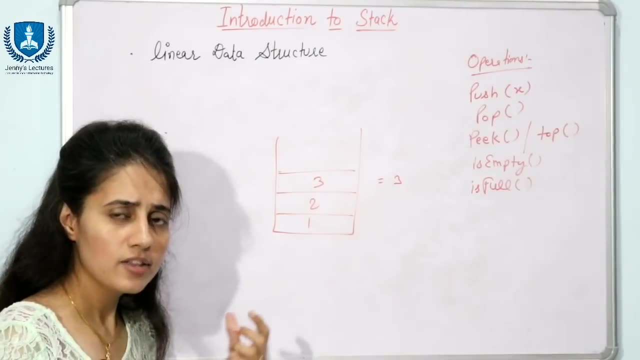 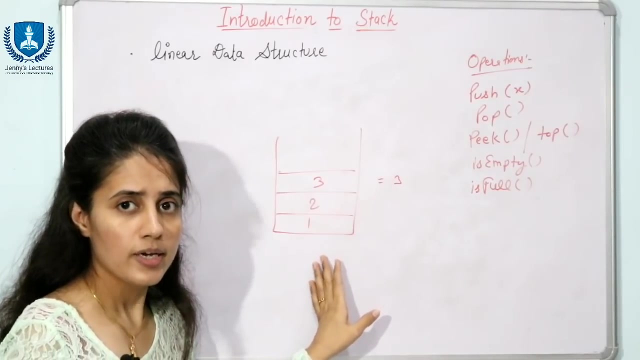 things like these. various operation works. you can perform search operation, traverse operation. you can find out that minimum element from the stack, maximum element from the stack right. that thing also we will discuss in later videos. right, these are some fundamental operations you can perform on stack. fine, now we will see the. 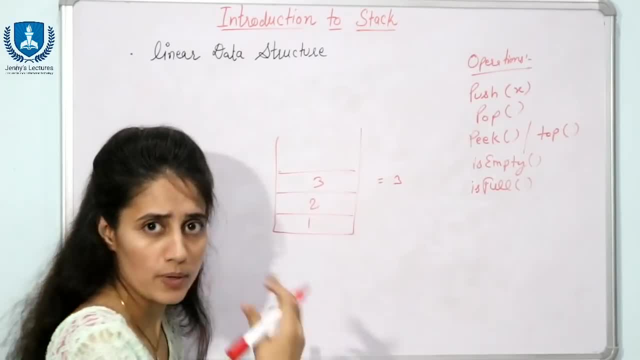 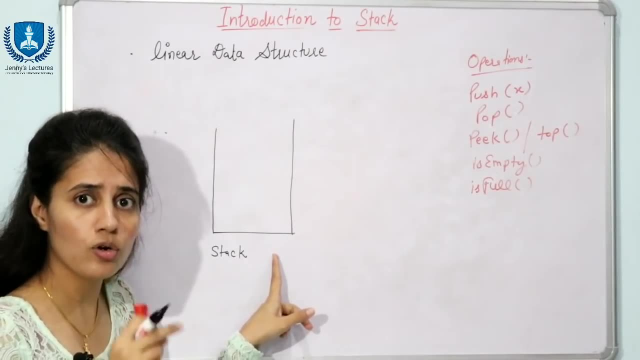 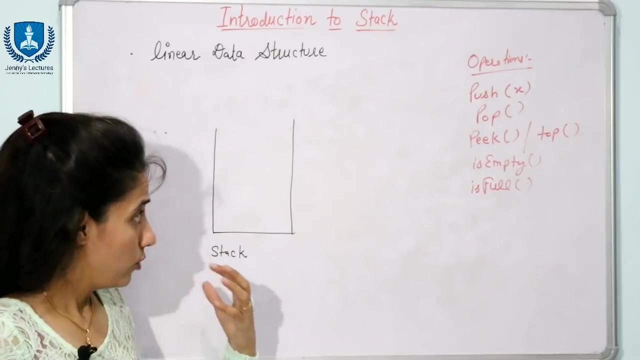 logical representation of stack as well, as we are going to perform these operations right. so this is how we logically represent the stack, right? not actually in the memory. this is just a logical representation, right for your understanding purpose. now, obviously, you want you want to push some data in the stack, right? so you need to know the capacity of the stack, or you can say the size. 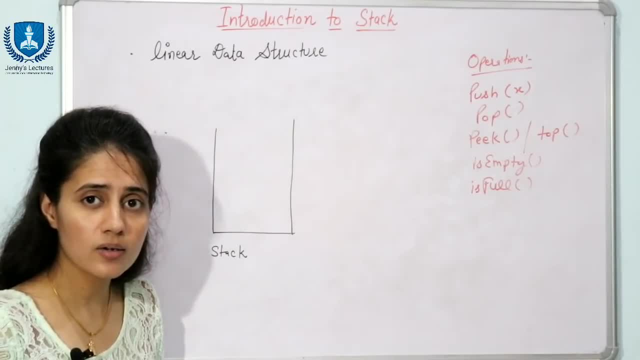 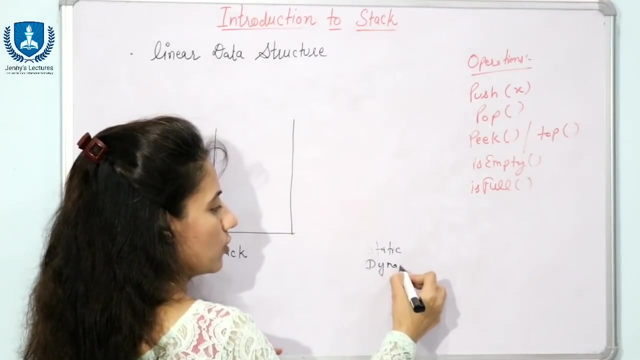 of the stack. so you need to allocate some memory to the stack, right, and how to fix that size, how you will get to know the size of the stack. you can allocate the memory either using static memory allocation or dynamic memory allocation. there are, there are, there are. 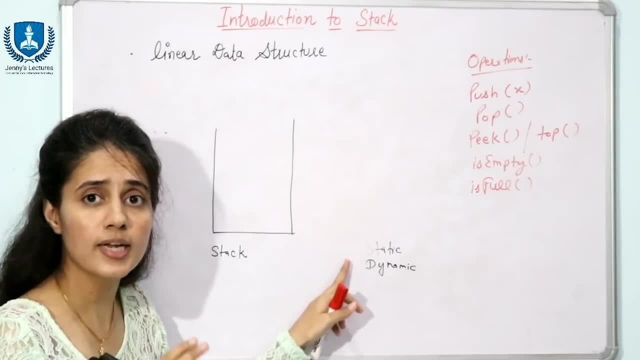 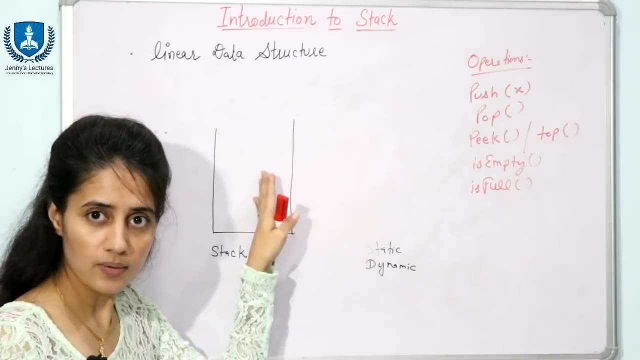 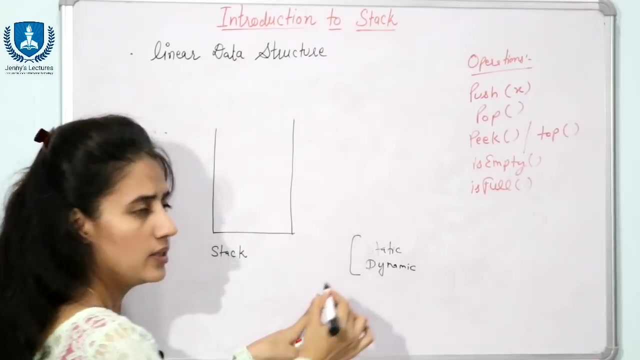 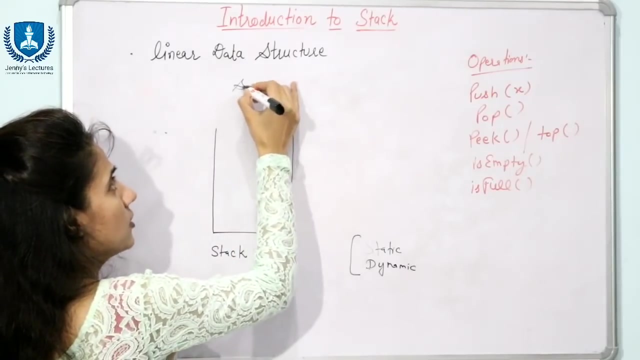 two ways to implement stack: static memory allocation and dynamically. you can implement stack. static means using arrays. you can implement stack right. dynamic means using link list. you can implement stack. so these implementations we will see in the next video with the proper, with the help of an example plus code right. so now suppose i have taken the size of the stack as five. 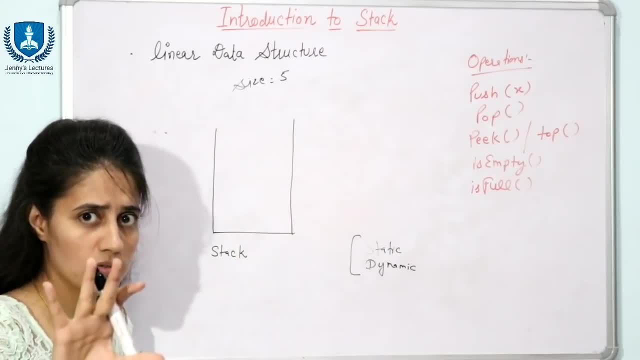 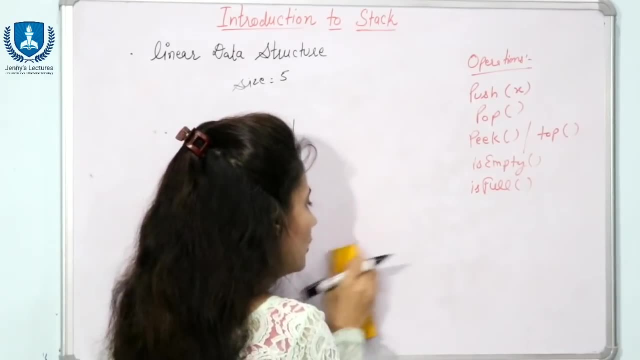 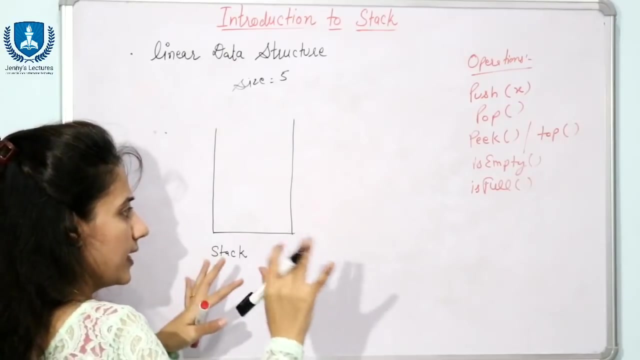 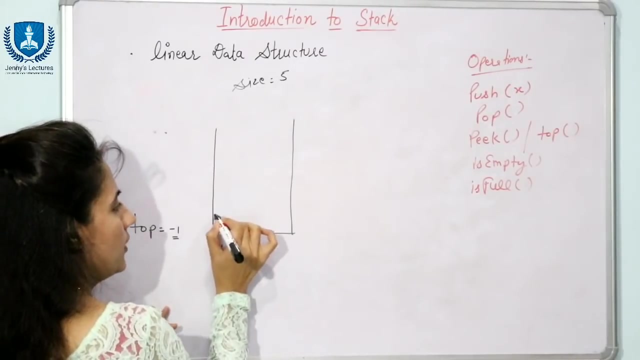 means the stack can store only five elements, either using by static memory location or dynamic memory allocation. right, that thing in detail we will discuss in next video. see, suppose the capacity is here five, so you can insert here five elements only. fine at starting, at starting top is what top is equal to minus one. fine, five means. 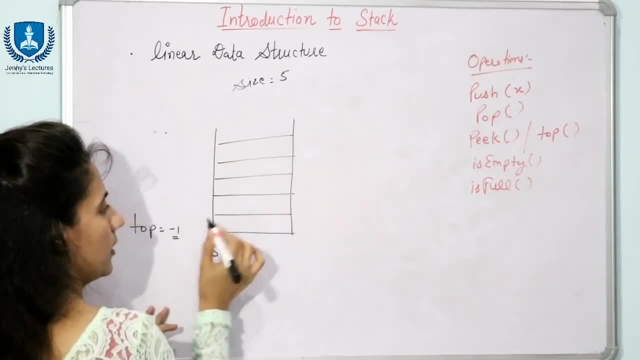 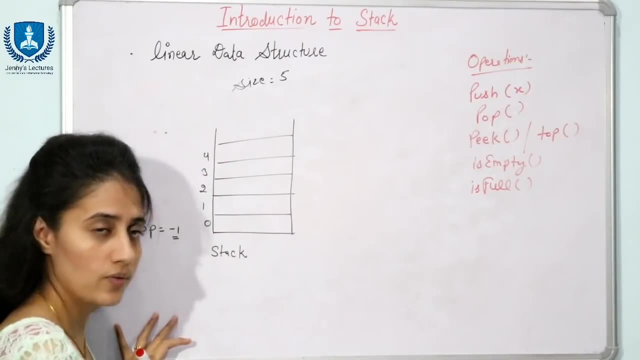 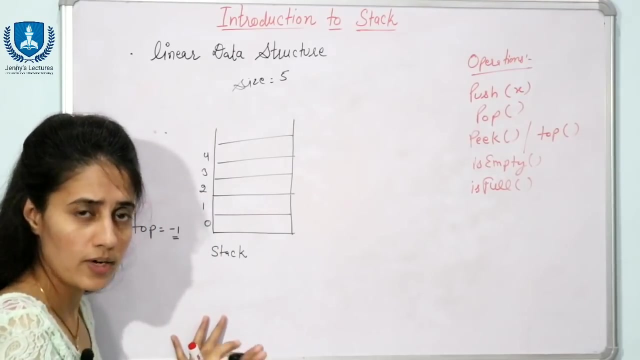 you can say you can insert five elements. the index would be zero first of all, then one, then two, then three, then four, from zero to four right. so here five elements i can store. this is the capacity of the stack. at starting top is minus one right. minus one means somewhere here. hypothetically we assumed this meaning. here there is minus one index. 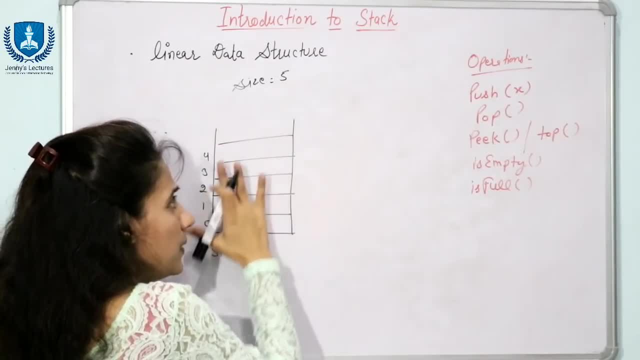 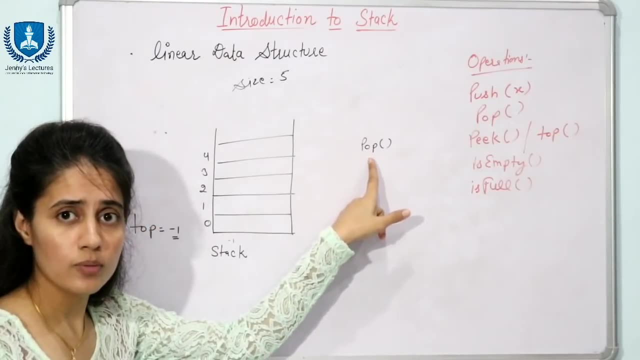 right now. suppose in the empty stack you called this pop operation, delete. now, Suppose in the empty stack you call this pop operation and if you keep in mind right, the top would be minus one dt. what would happen? pop means the topmost element would be removed, but here we don't have anything. 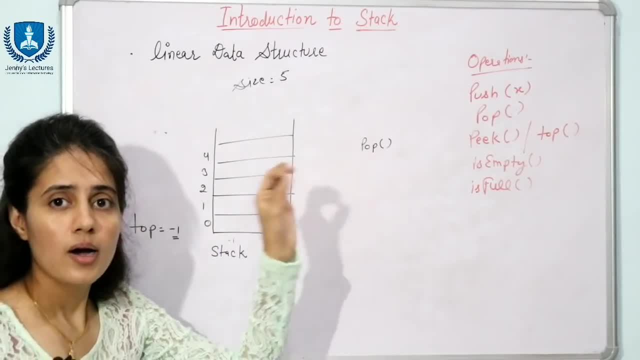 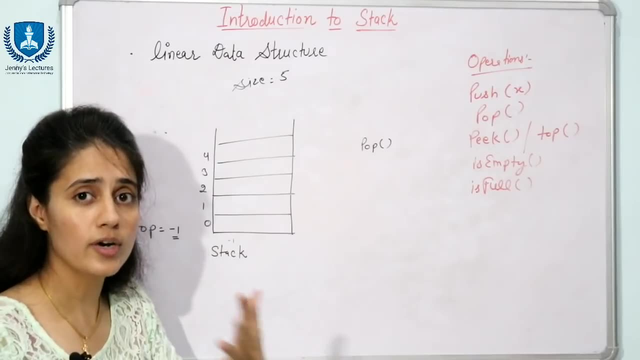 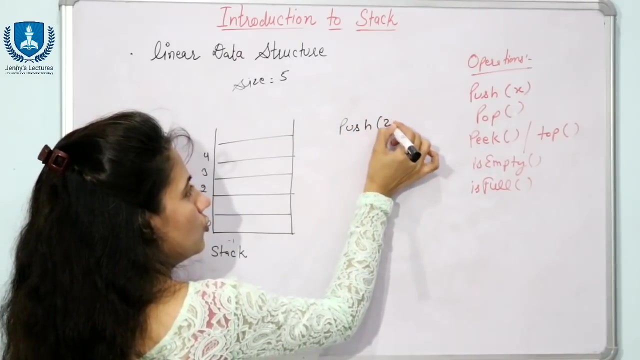 stack is empty. in this case it is what under flow condition it will return what the stack is empty. so this is what an under flow condition you can say right. and now suppose i am calling push two right actual implementation. also, we will see how to write down the code for push and pop. 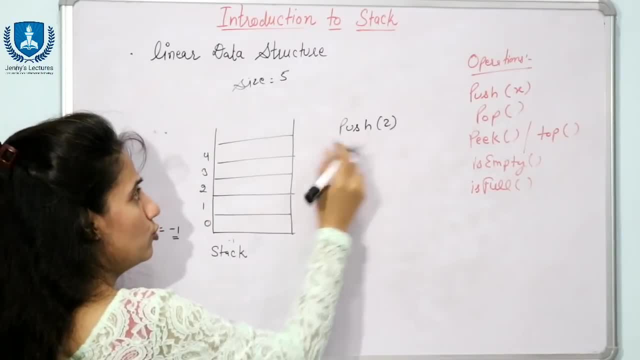 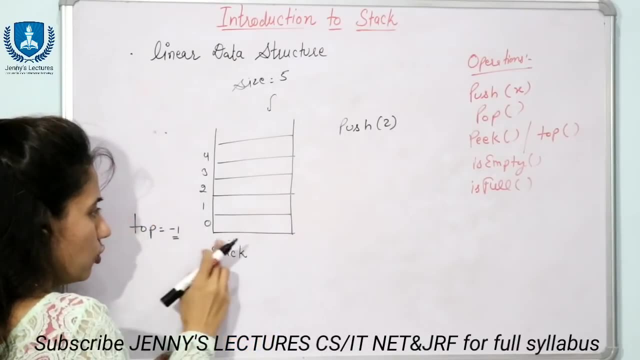 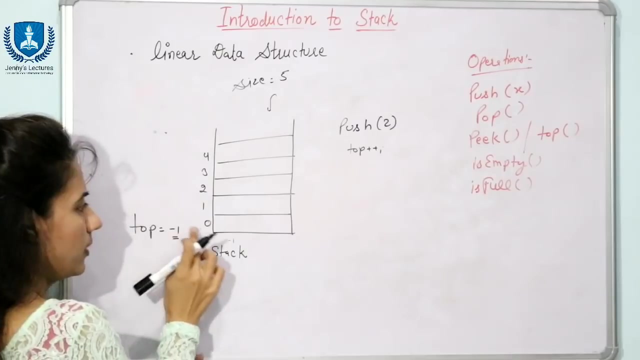 right here i am just giving you the brief introduction. push two means here, from the top only. you will insert this two right, we have only one end. so first of all, what would happen? top is minus one, so we will increment this top. first of all, top plus. plus. it means top becomes. 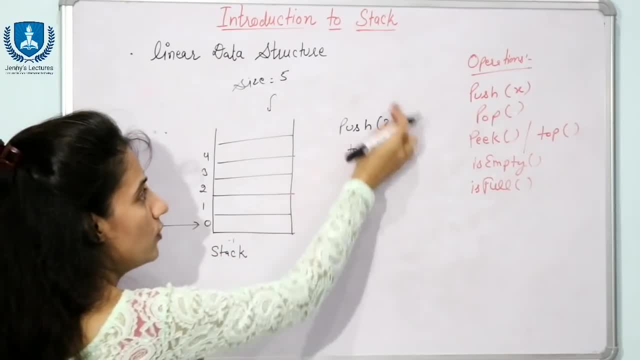 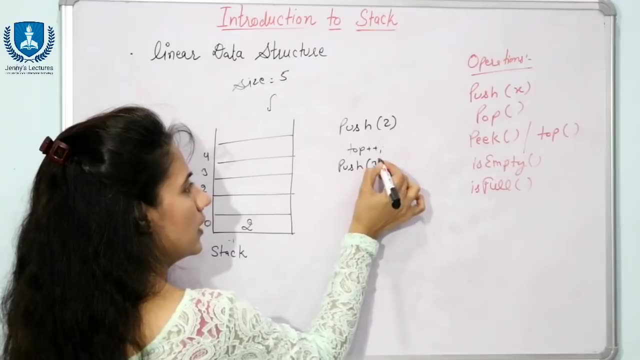 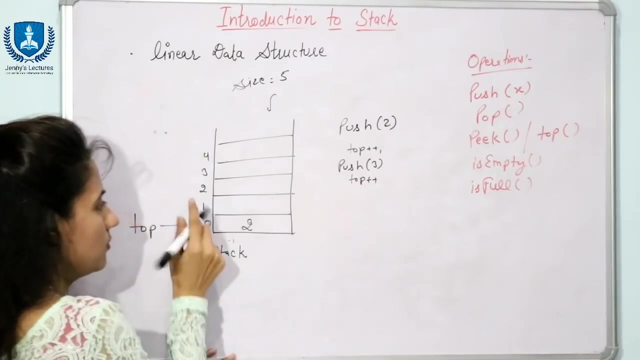 zero. now. now, here we have top, and now you will insert this two. you right again, if you will call push three again. first of all, top plus plus. right now top becomes this one. top is pointing to this one, one, and now you will insert three here in the 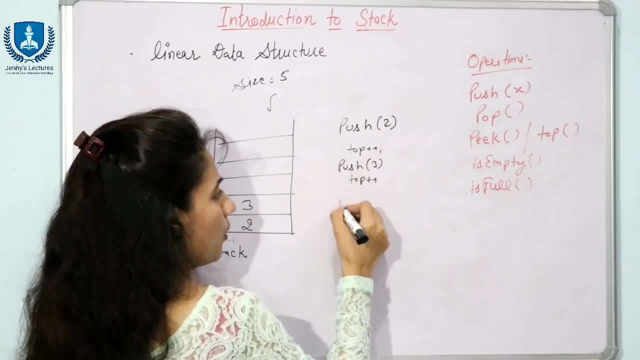 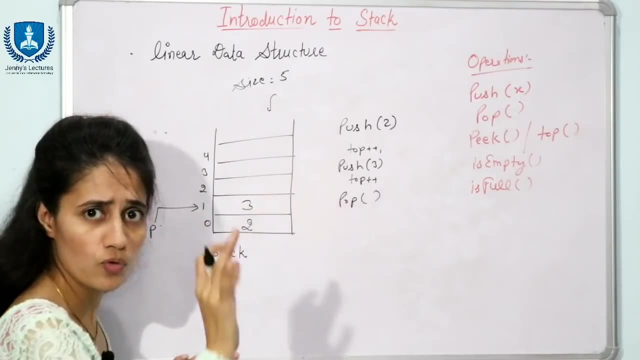 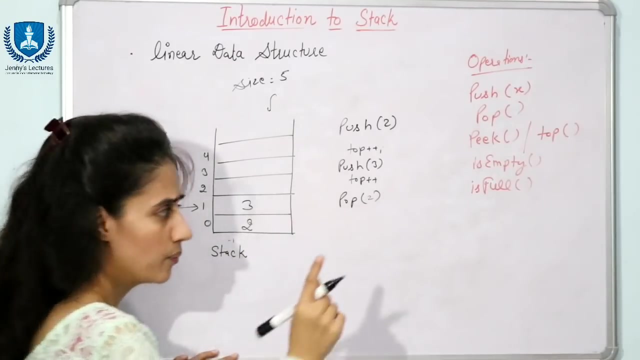 stack. fine, if you call pop no, need to pass any argument here. why so? because only the top most element would be removed from the stack. you cannot write here: pop two means if you want to remove this two, you cannot see pop two and this two would be removed. no, always this element. 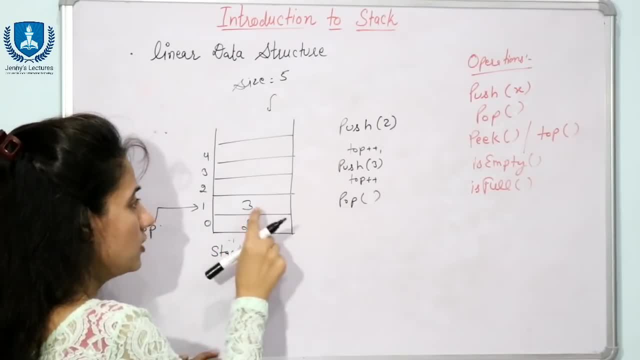 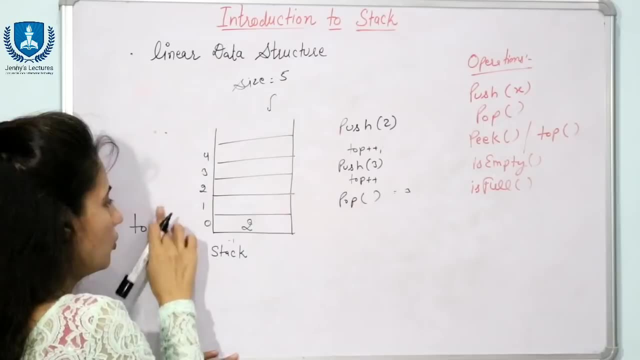 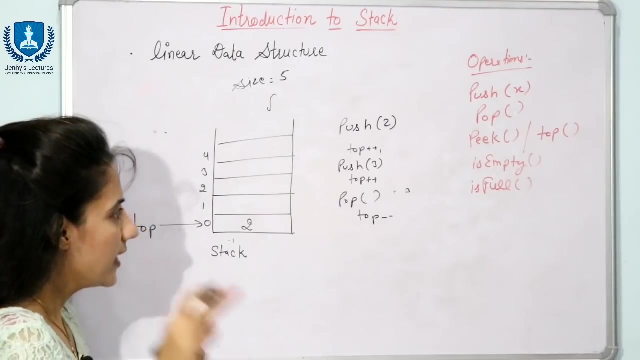 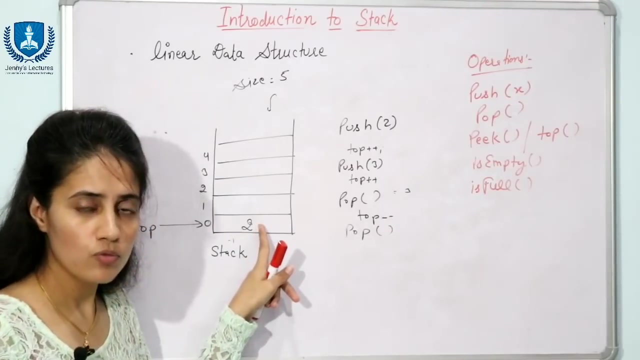 would be removed, right, so pop three. pop means the three would be removed from the stack. and now see, right now we will do top minus. minus means now again top is zero or second again. if you do do do to pop, in that case again two would be removed from the list. 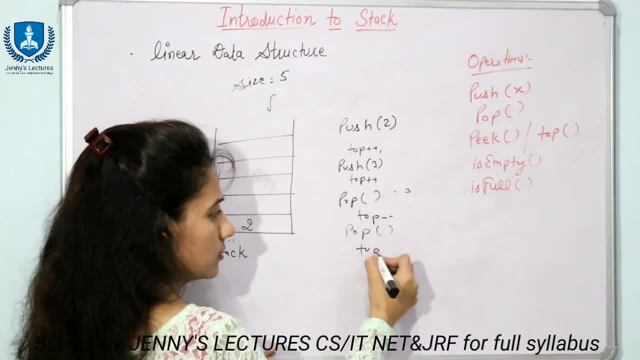 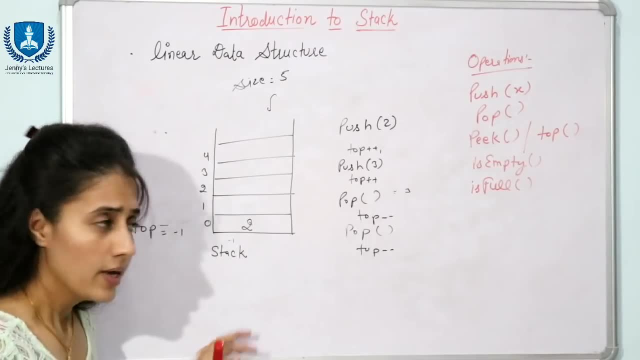 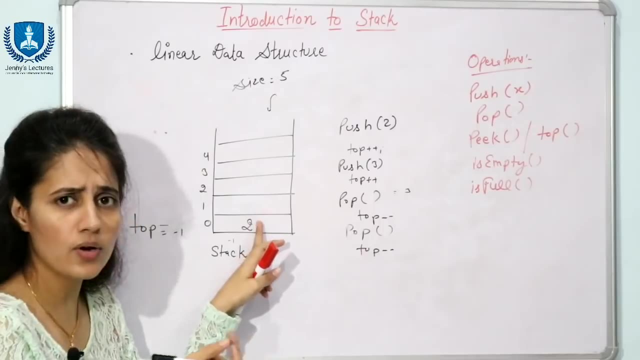 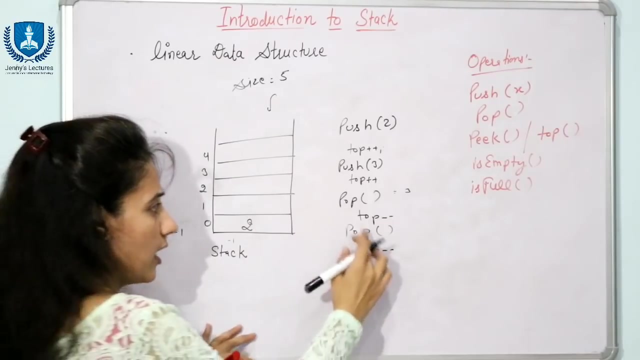 or simply you can do top minus. minus means top is now minus one right. and if you will not remove this, if you will not take out this from the stack, that is also fine, because this is now a garbage we do. we do not care what garbage value is there in the stack, because after 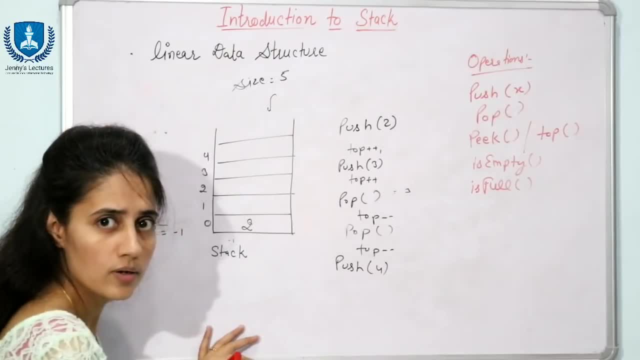 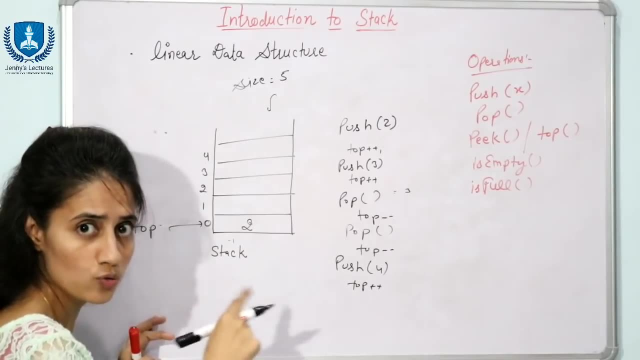 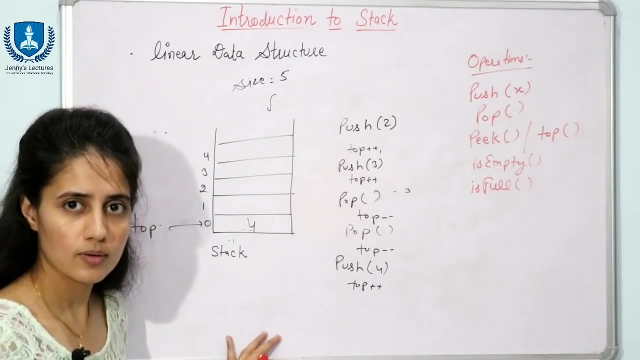 that if you will again call push four, then first of all top plus. plus means now top becomes zero minus one to zero. and here we will this: two would be overwritten and here four would be stored. right, this thing also. we will discuss how to code push and pop operation. fine, now suppose i have. 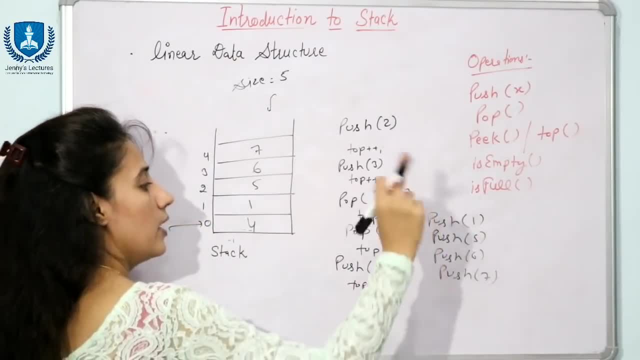 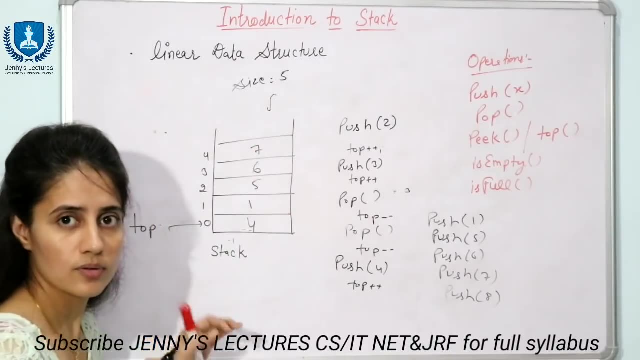 code: push four times one, five, six and seven. one, five, six and seven again. i am calling push eight right, and i am calling push eight, and i am calling push eight and i am calling push eight and i am calling now. the stack is full because capacity is only five right, so now it should return what it is, what. 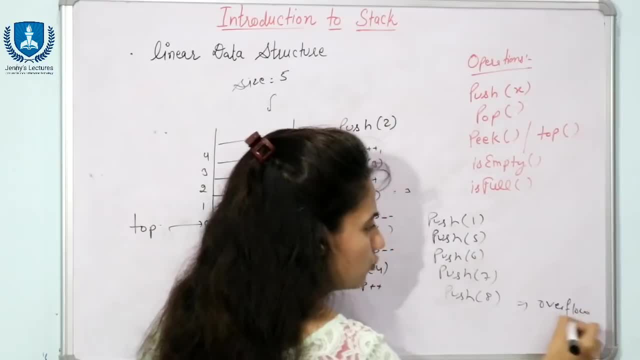 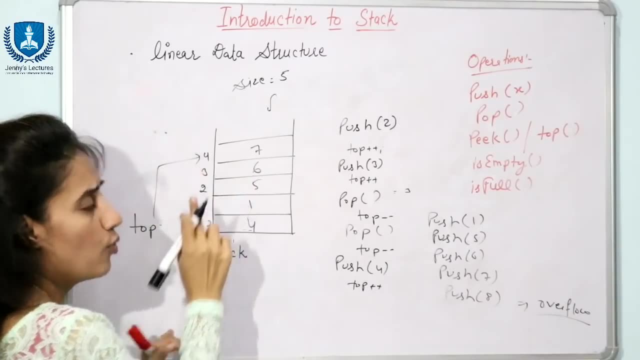 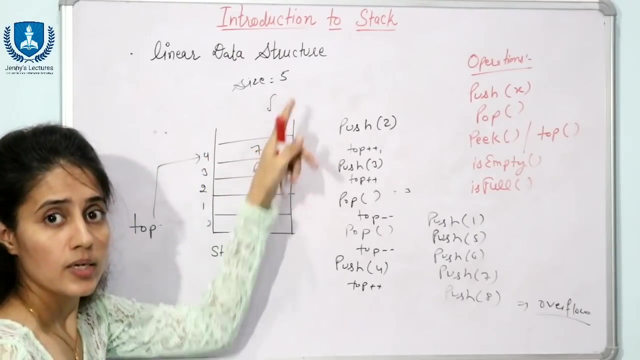 an overflow condition. we have discussed what is under flow condition now here. this is what overflow condition. if this top is pointing to this maximum size minus one, the index is four. maximum size is five. in that case it would return overflow condition. you cannot insert any data in. 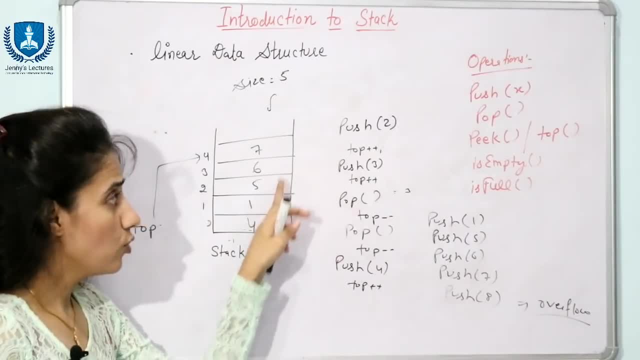 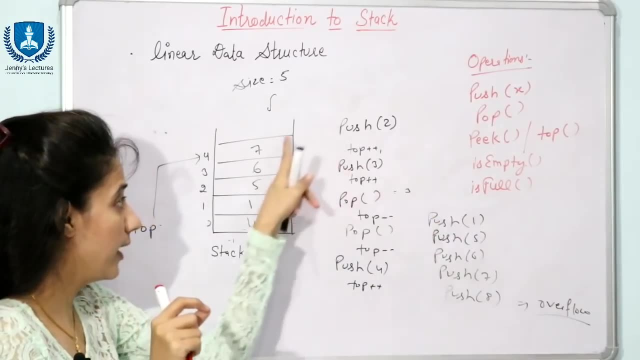 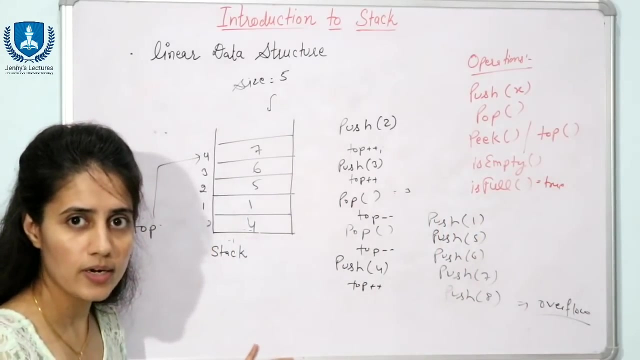 the stack because stack is full. so this is what overflow condition- and now here, if you will call, is full function means it will return true if the stack is full. and now the condition is stack is full, so it would return. at this time is full function would return true, right and when there. 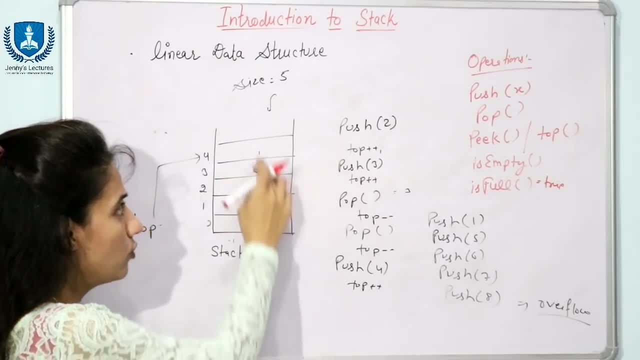 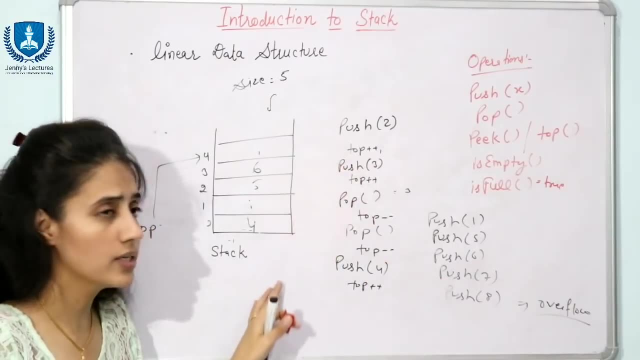 is nothing in the stack. suppose we have popped out all the data and after that we call is empty. in that case it would return true, because stack is empty. how you will? you are going to code these function. we will see, fine. so now, what are the applications? 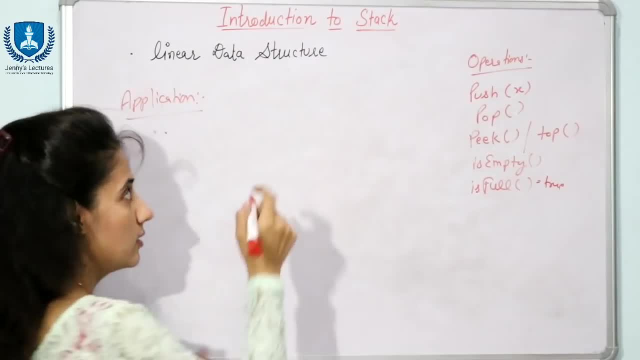 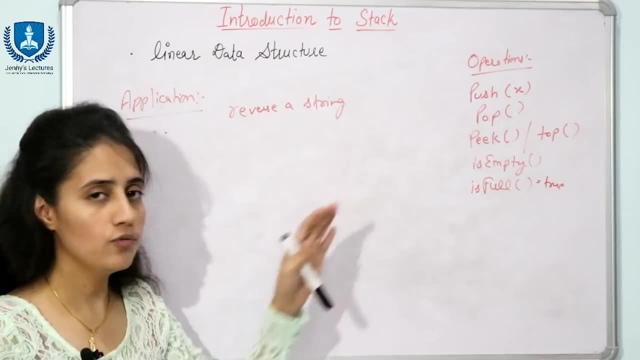 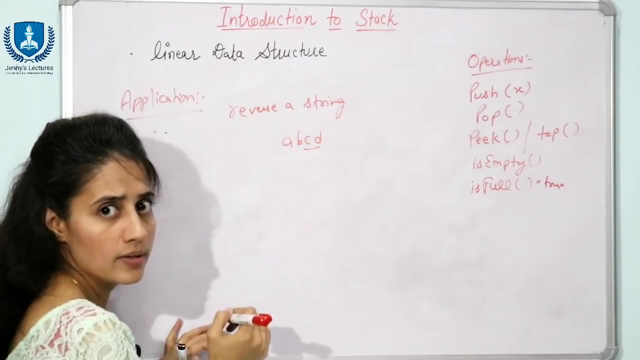 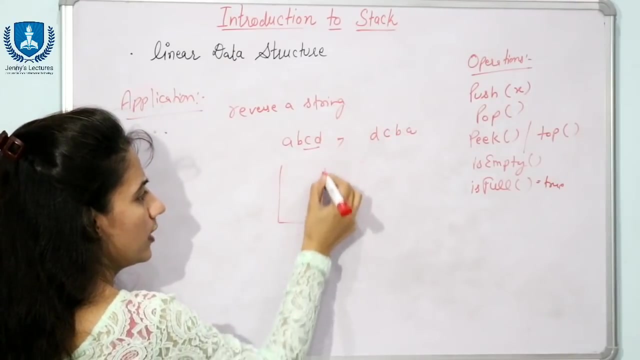 of stack. see, the very basic application is: if you want to reverse a string or reverse a word, then we will use stack. that is very simple. suppose i want to reverse. i have a string a, b, c and d, so i want to reverse this. i want to print d, c, b and a. so simply, what i can do, i can push. 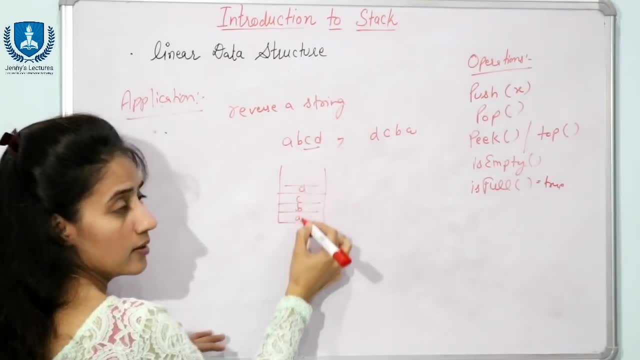 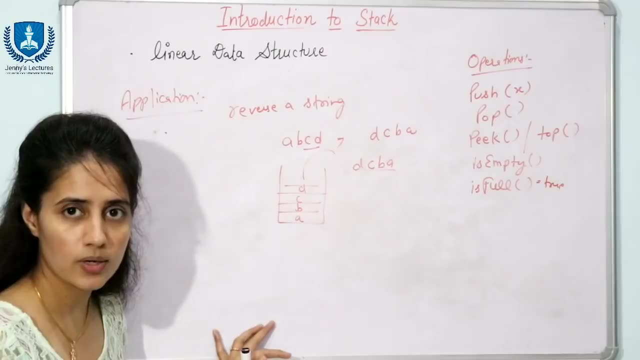 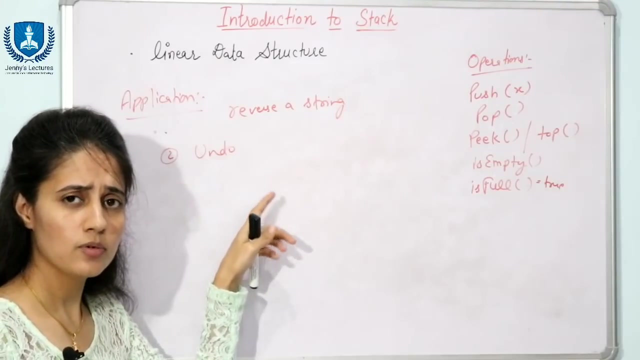 this into stack: first of all a, b, c and d and then pop out. first of all d would be popped out, then c, then b, then a. this is what we have reversed. the string second application is for undo mechanism in text editor. i guess everybody have used this undo mechanism. suppose you have written something. 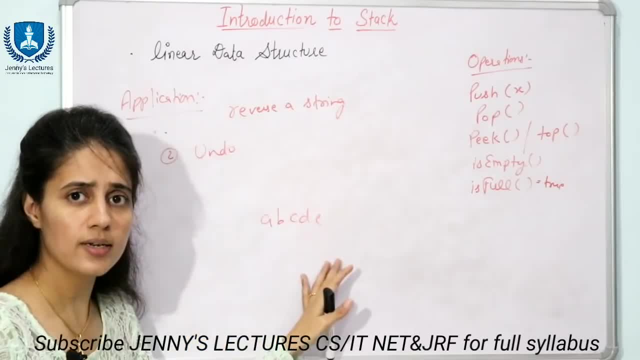 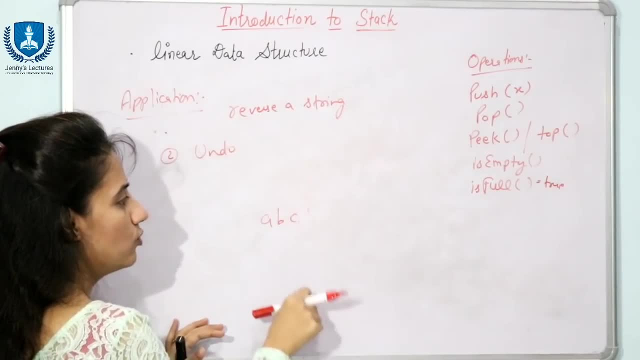 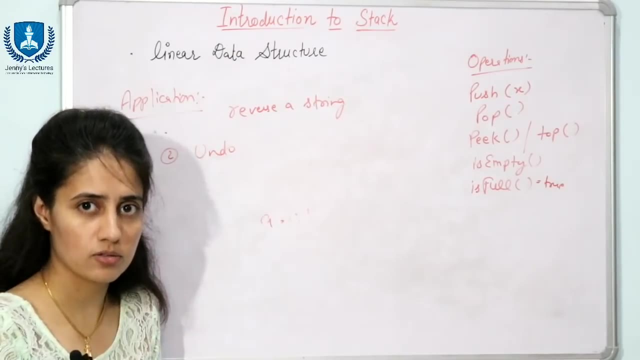 i have written a, b, c, d, e right in the text editor and in text editor and when you press ctrl z, the shortcut key for undo, then e would be deleted, then d would be deleted, then c, then b, then a. this mechanism is performed using stack in your text editors. 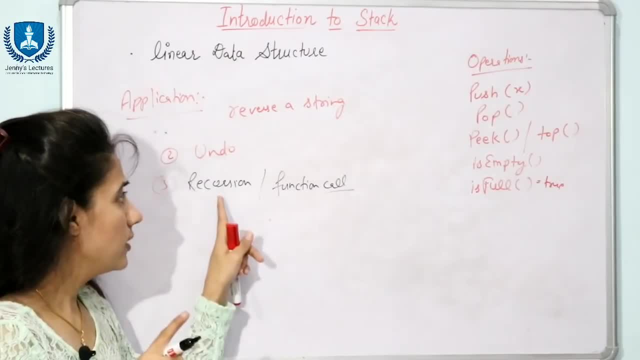 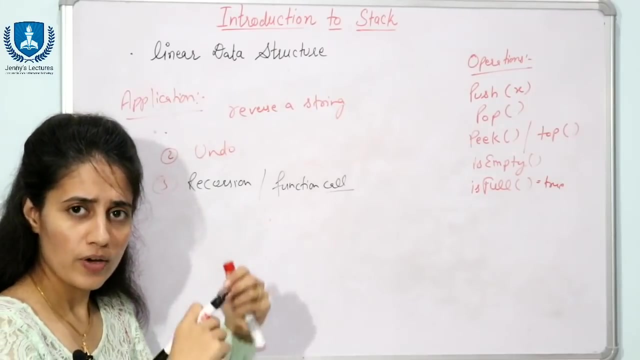 right. third application: maybe you can use it in recursion or you can say in function call. when you are going to call a function, then obviously something would be returned, some value would be returned like, and recursion means it is, you can say, a chain of function call. a function is calling itself again and again, right? so whenever that function would